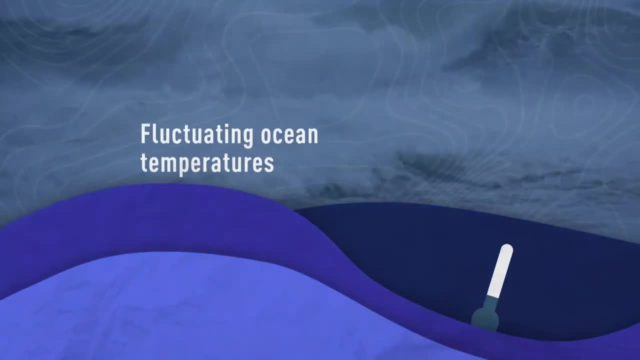 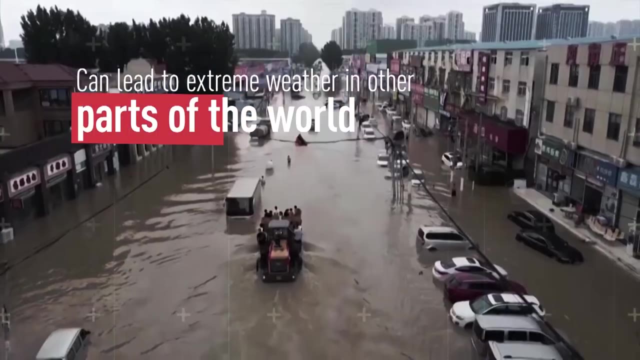 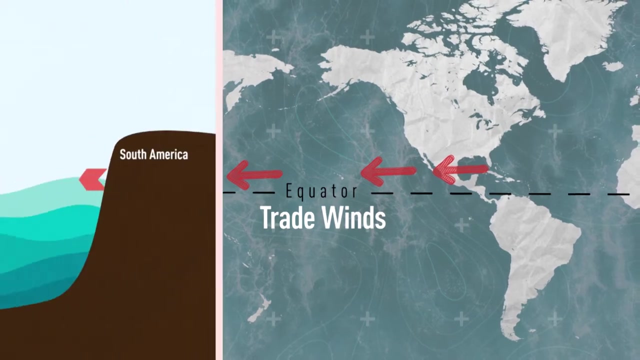 These weather patterns occur as a result of fluctuating ocean temperatures in what is called the East Central Equatorial Pacific Ocean, but it can also lead to extreme weather in other parts of the world. During normal conditions in the Pacific Ocean, trade winds blow west along the equator, taking 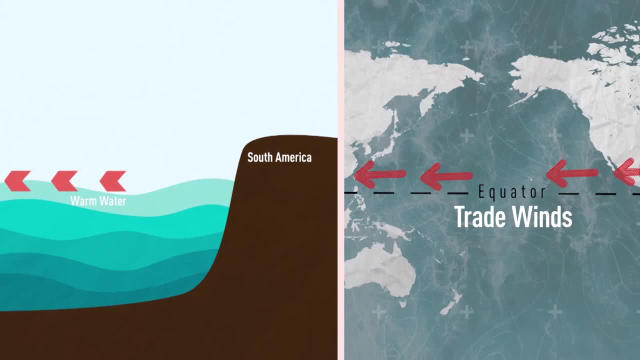 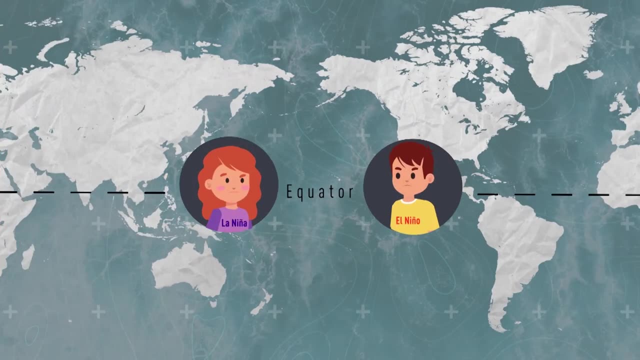 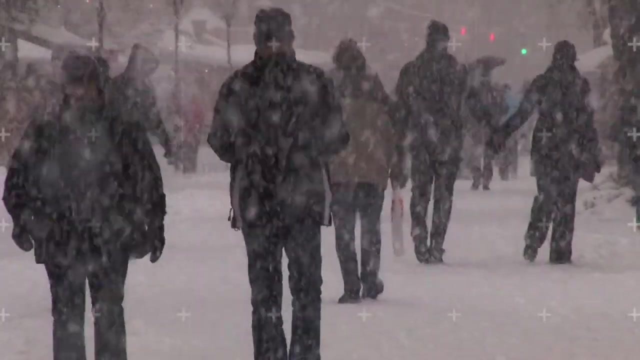 warm water from South America towards Asia. To replace it, cold water rises, a process called upwelling. El Niño and La Niña change all that. If a winter is the opposite of what you'd expect, it's likely because of an El Niño. 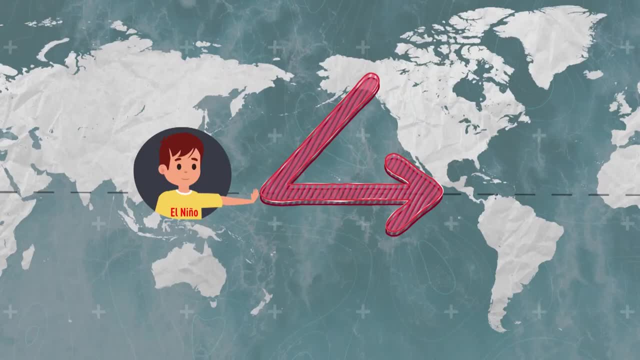 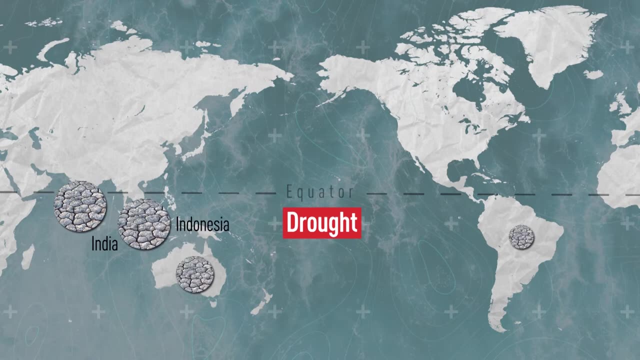 event El Niño weakens trade winds. It's a sign of a drought pushing warm water back east, towards the west coast of the Americas. Chances of drought increases for India, Indonesia, Australia and a large section of the Amazon. 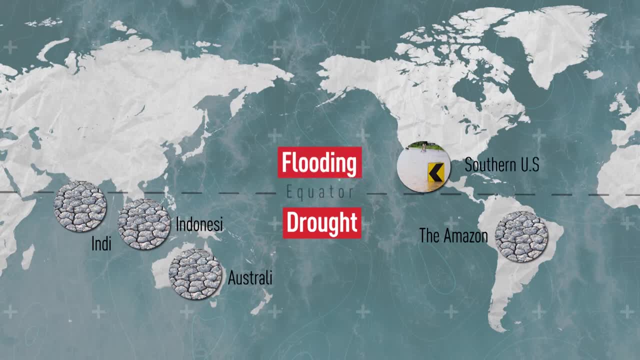 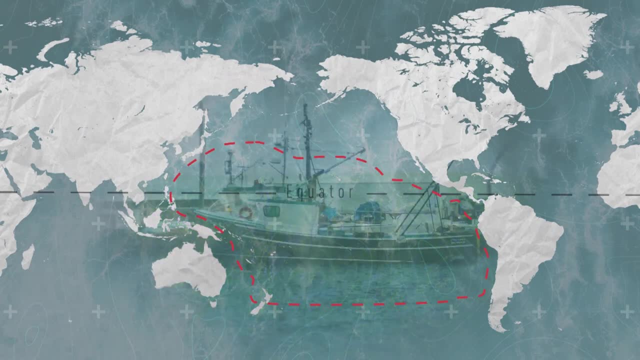 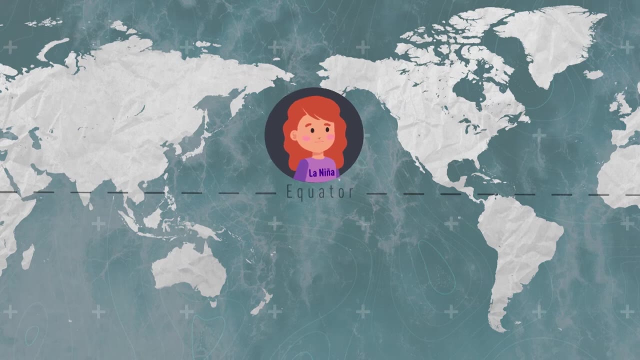 with the southern US experiencing increased flooding. El Niño mostly affects developing countries bordering the Pacific Ocean which depend on agriculture and fishing. El Niño's sister, La Niña, effectively argues with her brother and does the opposite: She cools the ocean surface temperatures, bringing wetter conditions for the same parts. 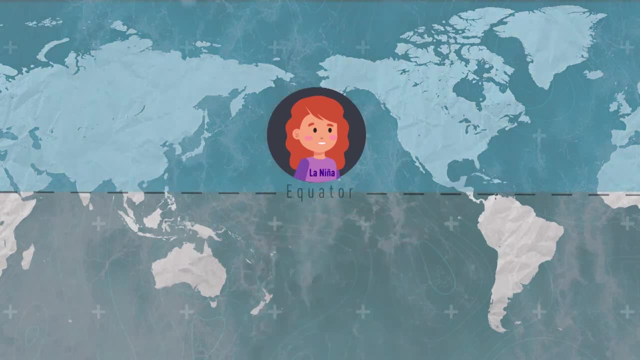 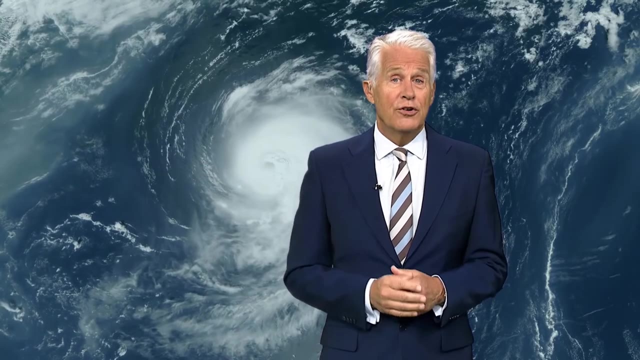 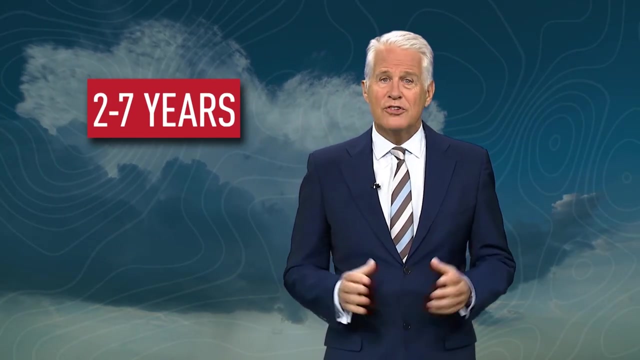 of the globe Now. a La Niña year means colder winters in the north and milder winters in the south. She can also cause a more severe hurricane season. Episodes of El Niño and La Niña tend to happen every two to seven years, and typically. 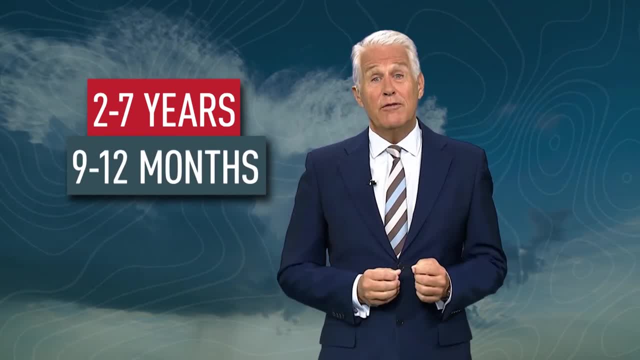 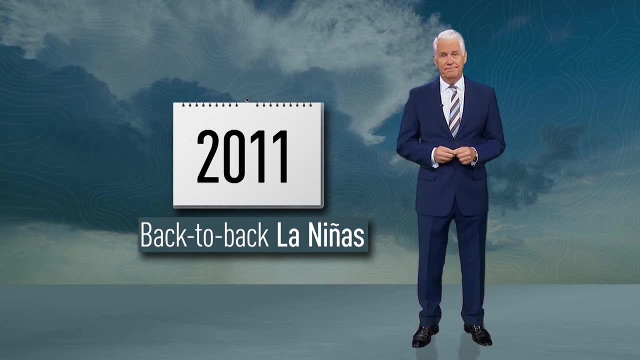 last between nine and twelve months, but can sometimes stay even longer. There were back-to-back events. There were back-to-back events. There were back La Niñas in 2010 and 2011.. Advances in technology are helping some countries predict, respond and adapt to the effects. 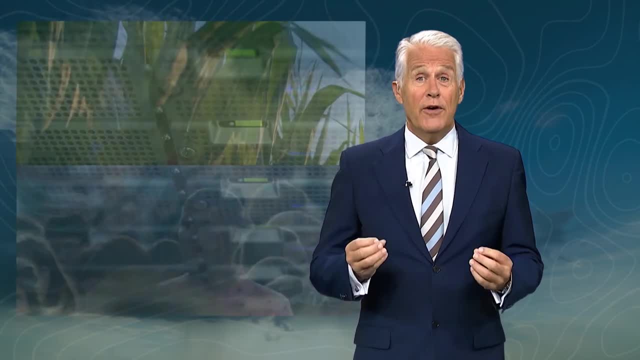 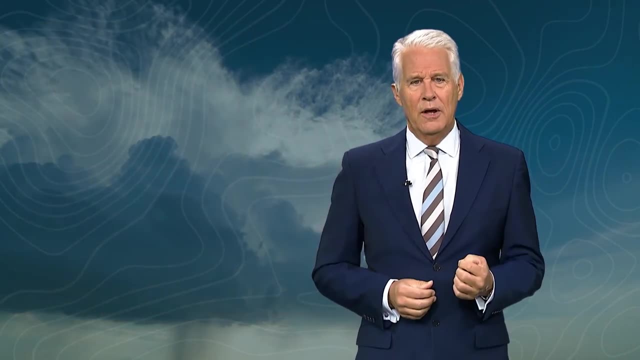 of El Niño and La Niña, often saving vital crops and livelihoods. Individual weather events, though, in their link to climate change, is one of the key issues on the table at the world's most important climate conference – COP26.. END.